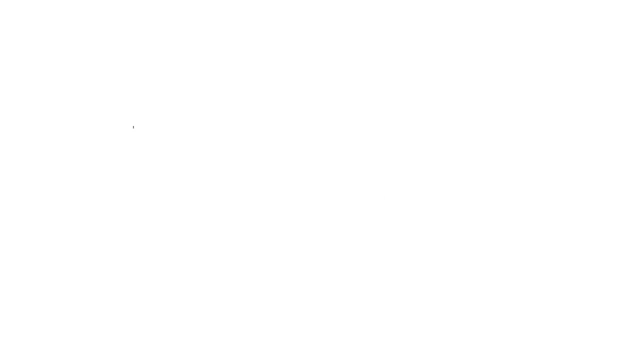 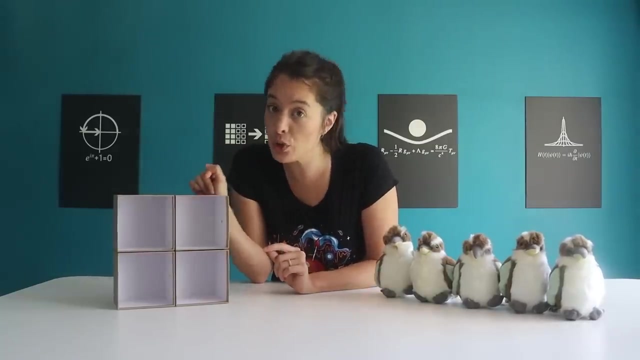 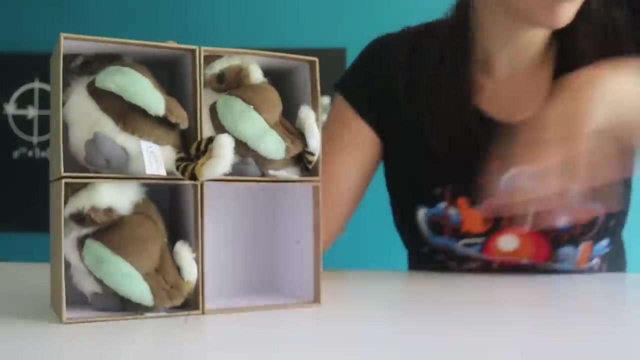 Thank you to Brilliant for sponsoring this episode. Hi guys, Jade here, Here's a super simple argument. If I have five Australian pigeons and four pigeon holes, if I want to put each pigeon into a pigeon hole, there must be at least two pigeons in the same pigeon hole. 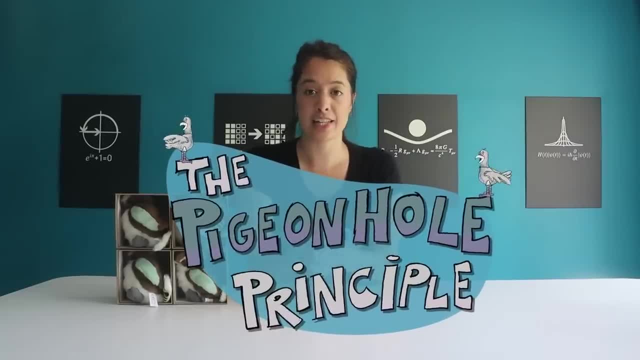 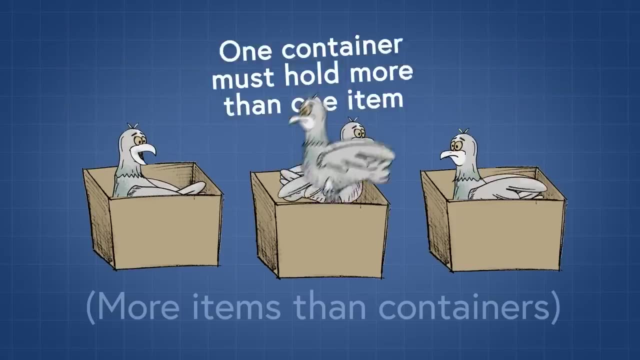 This is called the pigeon hole principle And more generally, it states that if you have more items than containers, if you want to put every item into a container, there must be at least one container with more than one item in it. So why is this even a thing? 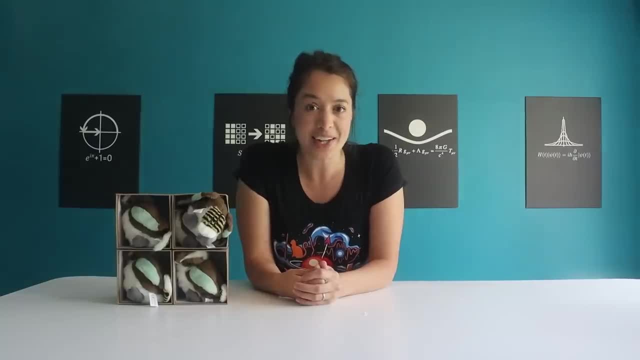 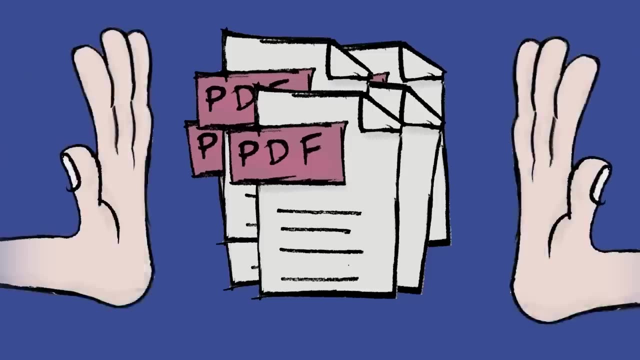 It's practically counting, But we'll see that it's surprisingly powerful. It can prove that in any big city, at least two people have the same number of hairs on their head. It reveals a fundamental limit of information- compression, and it can help prove that some infinities 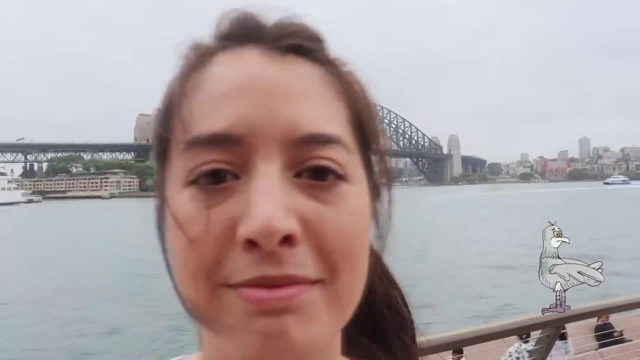 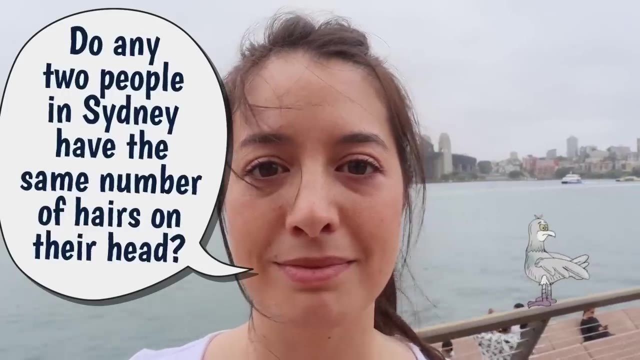 are bigger than others. If someone came up to you and asked: do any two people in Sydney, Australia have the same number of hairs on their head? What would you say? How would you even begin to figure it out? You might think you had to go around to every Sydney cider. 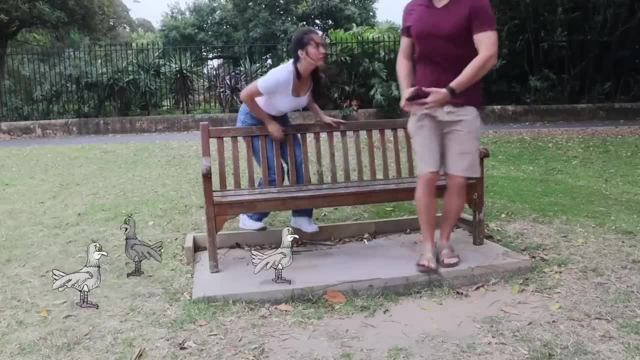 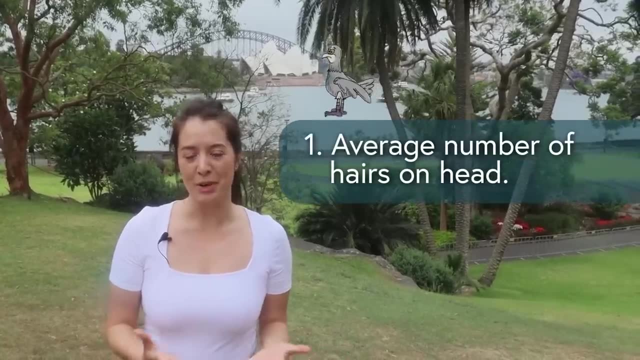 and count all of their hairs and then see if you found any two with the same number. But thanks to the pigeon hole principle, we don't need to do that. We only need to know two things: the average number of hairs on a person's head. 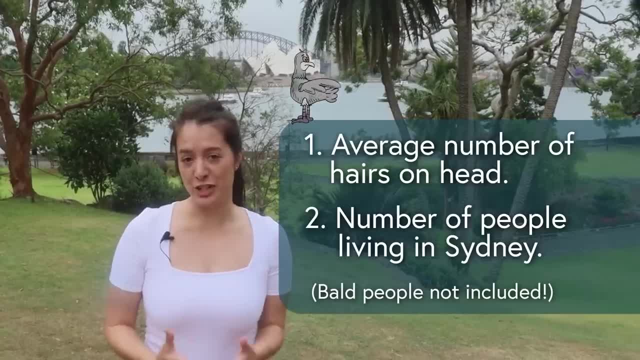 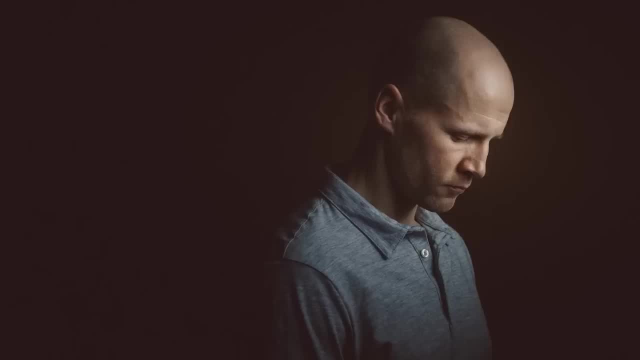 and the number of people living in Sydney. I should mention to make this interesting. we're going to leave out bald people who have zero hairs on their head, because obviously all bald people have the same number of hairs on their head. Sorry, bald people. 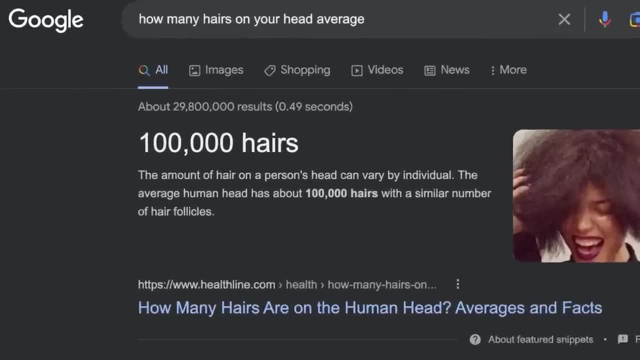 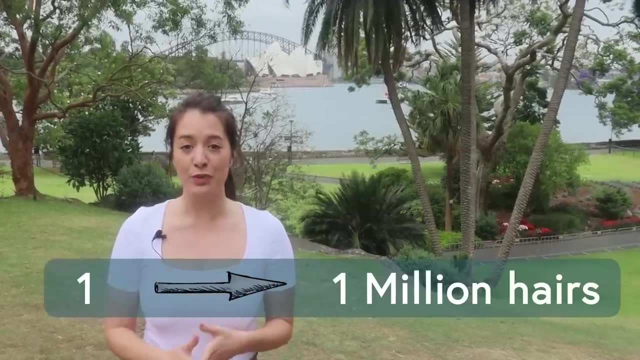 So what's the average number of hairs on a human head? According to Google, it's about 100,000.. We'll assume that no one in Sydney has more than one million hairs on their head. So we've got a range of one to one million hairs. 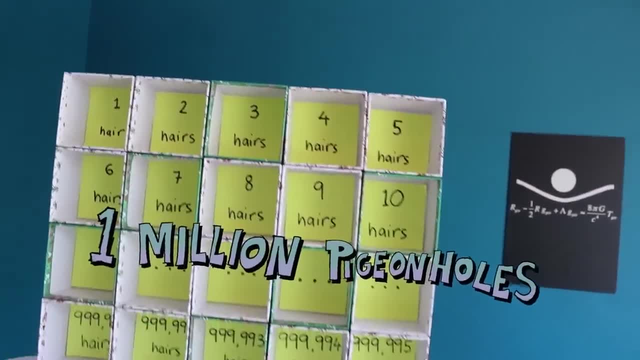 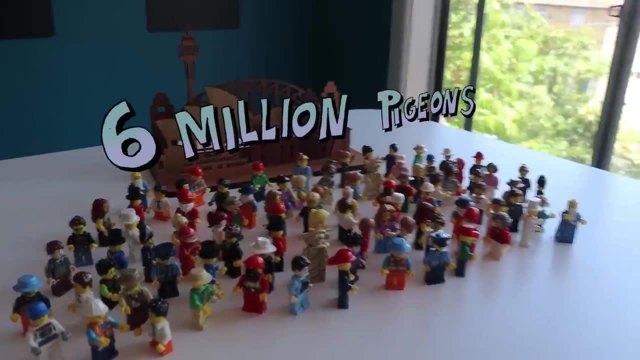 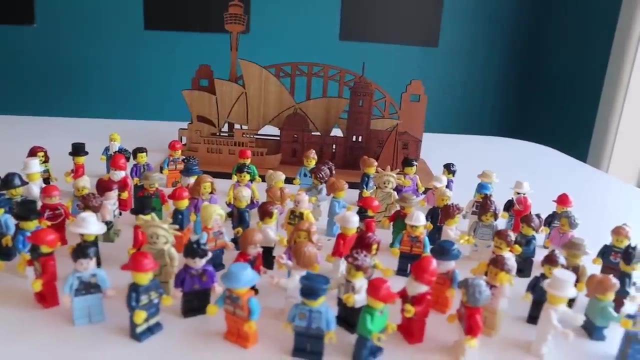 These will be our pigeon holes. The population of Sydney, Australia, is about six million. They will be our pigeons. Let's fill our one million pigeon holes with one million Sydneysiders. He has one hair, she has two hairs, he has three hairs. 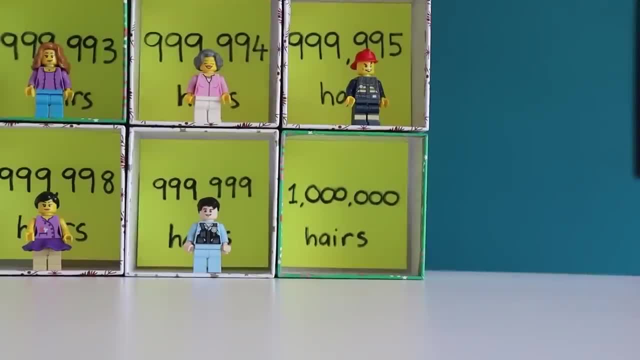 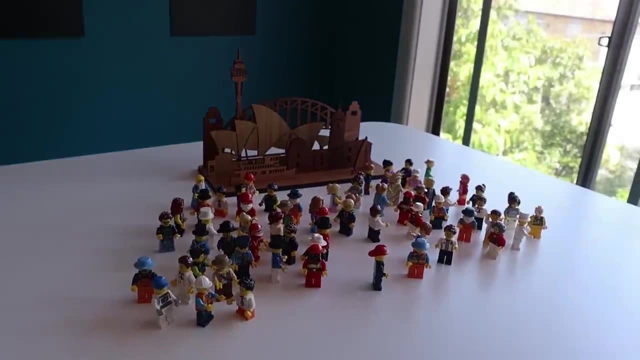 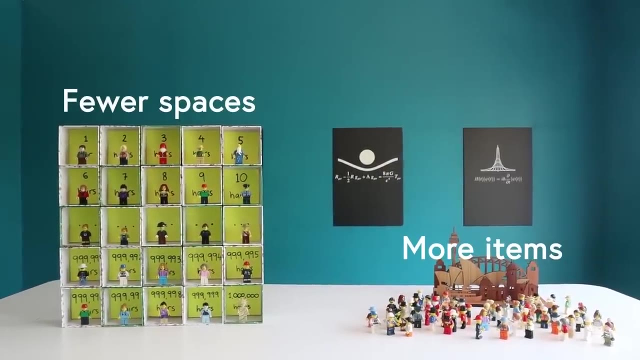 all the way up to a million hairs, We still have five million Sydneysiders left who need to go into a pigeon hole According to the pigeon hole principle, because the number of Sydneysiders is larger than the number of possible hairs on a human head. 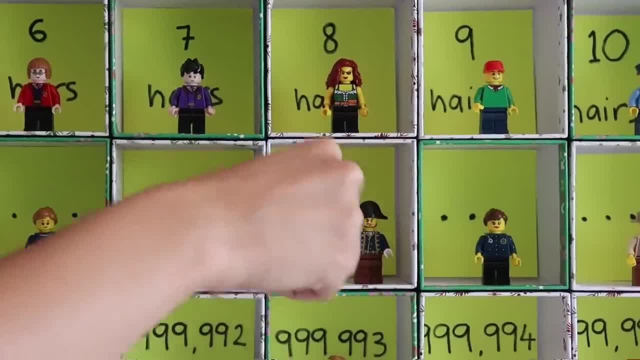 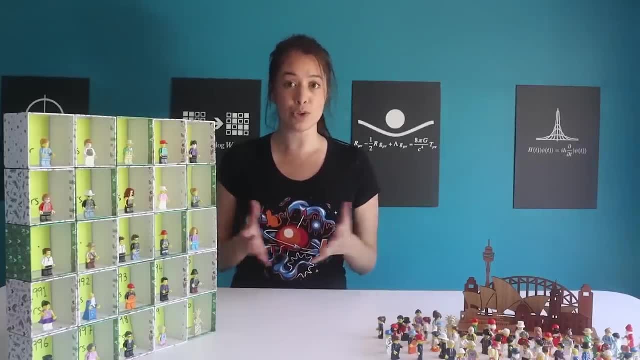 there simply must be at least two Sydneysiders with the same number of hairs on their head. This is amazing. Without having to know the actual number of hairs or the two individuals with the same number of hairs, we've managed to prove that in any city. 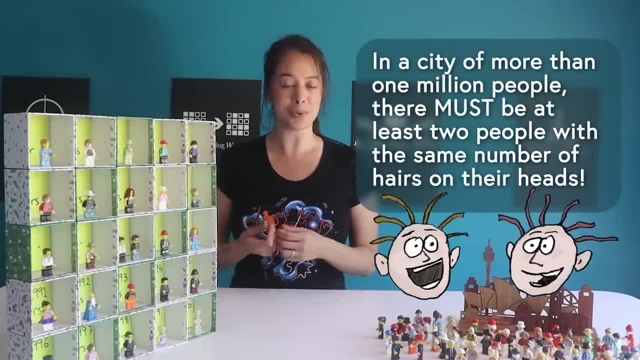 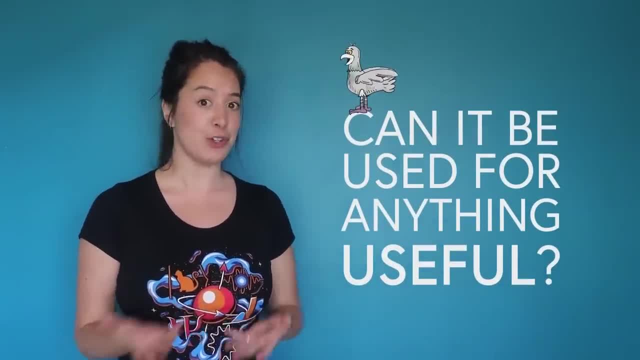 of more than one million people, there must be at least two people with the same number of hairs on their head. That was a fun but useless result. Can the pigeon hole principle be used for anything useful? Yes, it reveals a fundamental limit of data compression. 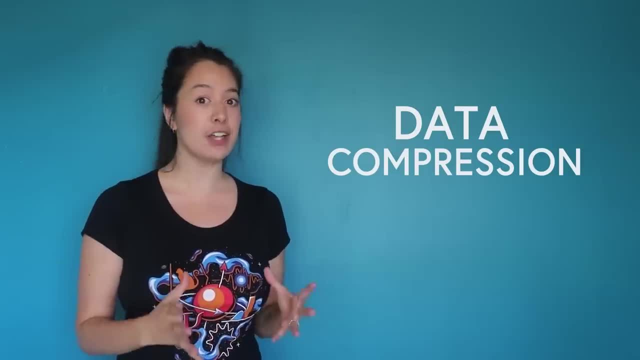 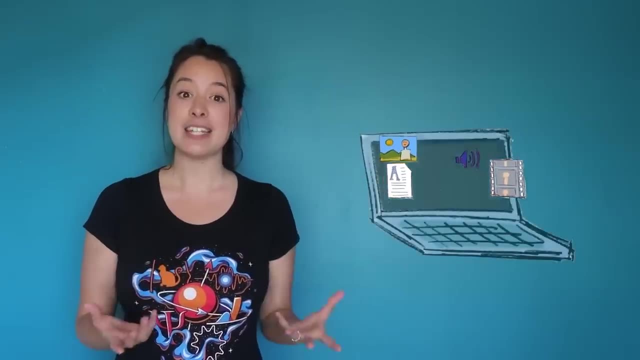 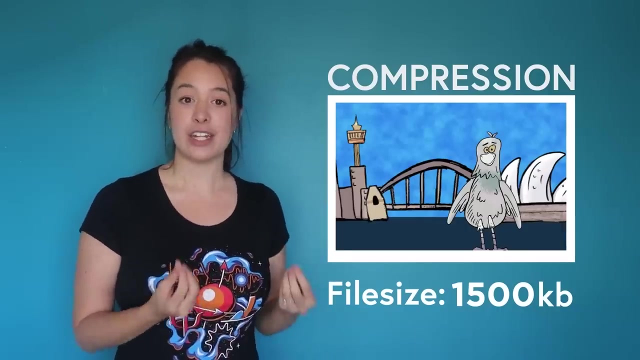 Data compression is the technique used in computer science to make large computer files, like images, audio and video recordings, into smaller files. This makes them easier to store on your computer or send over the internet. Data compression works by manipulating the data so that it uses fewer bits of information. 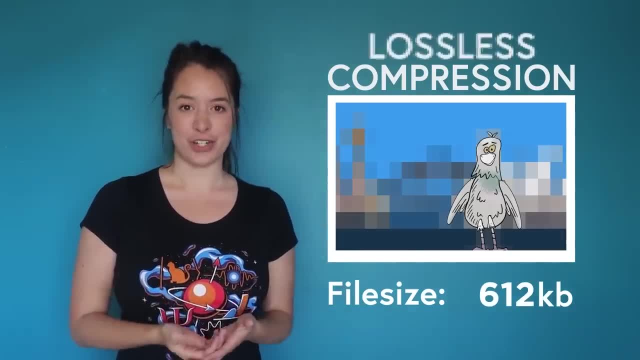 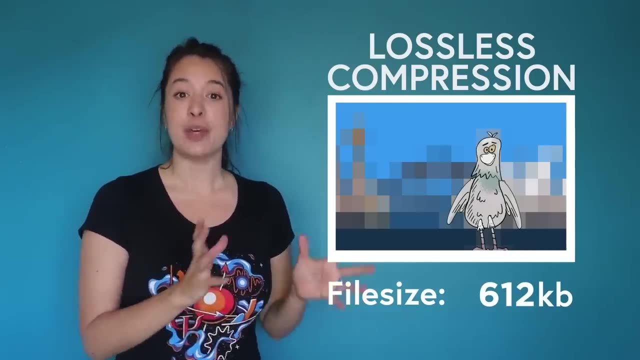 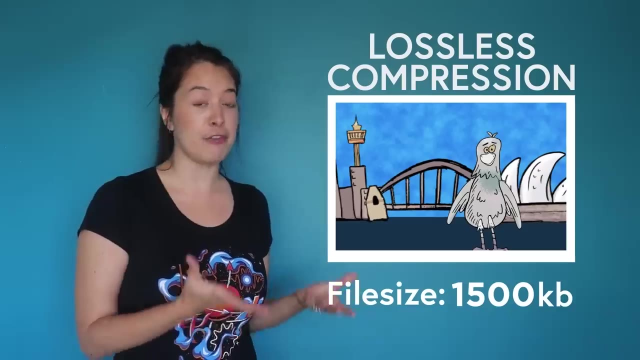 than the original file. A very common type of data compression is lossless compression, As the name suggests. no information is actually lost during this compression, and we can always get back all of the original data from the compressed data. How? How can you reduce the number of bits used to represent a file? 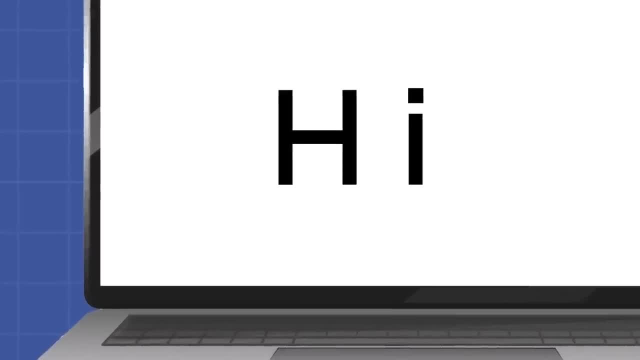 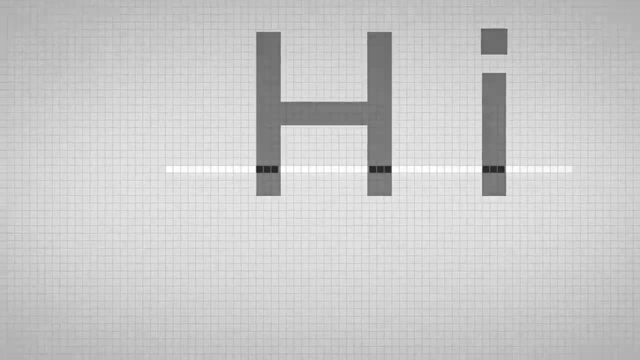 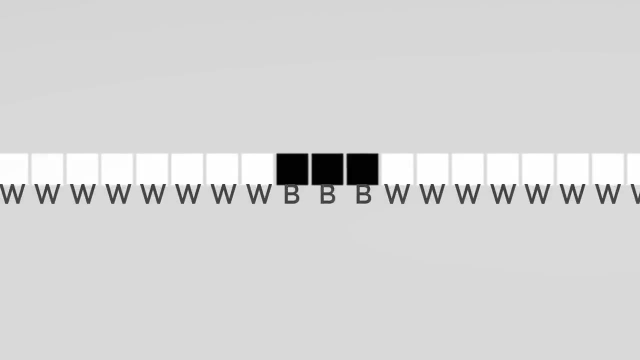 without losing any information. It's pretty interesting. Consider a screen of plain text on a white, solid background. There are many long runs of white pixels and many short runs of black pixels. A single line of pixels could be represented like this: a W for every white pixel and a B for every black pixel. 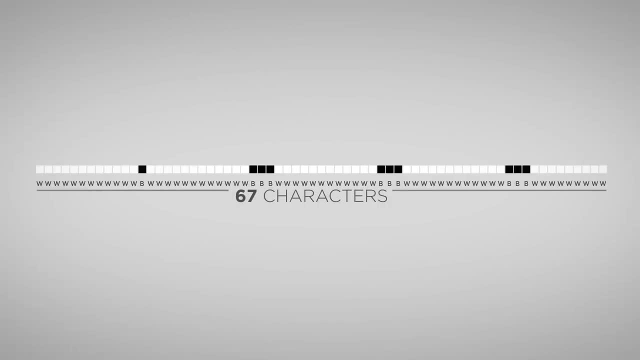 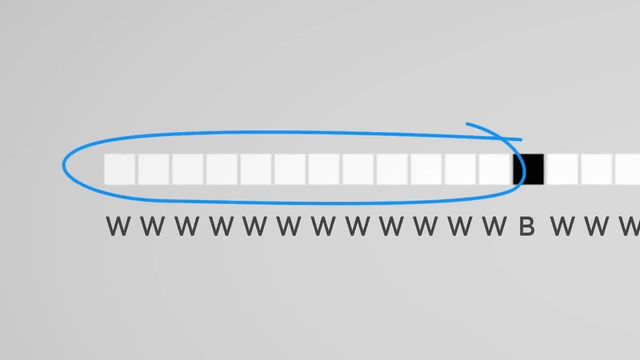 a total of 67 characters. Using a lossless compression algorithm, we can represent the same information more efficiently. Take this string of 12 W's. Rather than writing out each W individually, we can write a 12 and then a W to signify that there are 12 white pixels in a row. 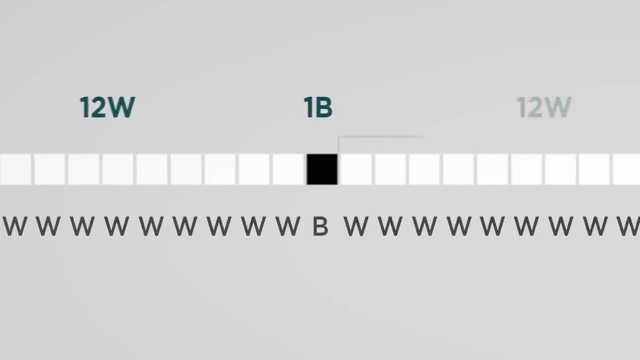 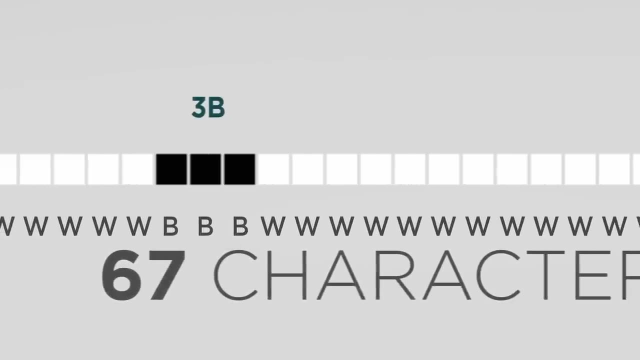 Similarly, we write one B to signify one black pixel, another 12, followed by a W to signify another row of 12 white pixels. three B for three black pixels, and so on, compressed, the original 67 characters down to just 18.. 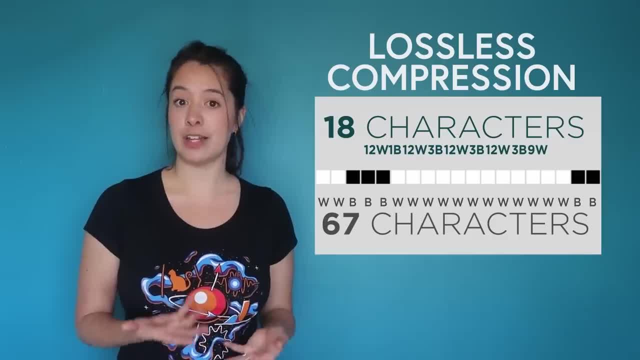 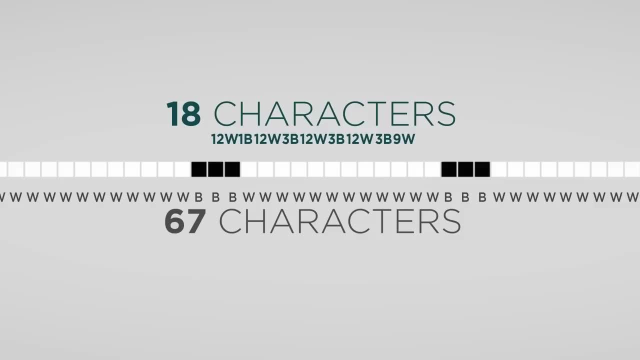 While the actual format used for the storage of files is generally binary rather than ASCII characters like this, the principle remains the same. If we want to convert the compressed data back to the original data, we can do so because no information is actually lost. 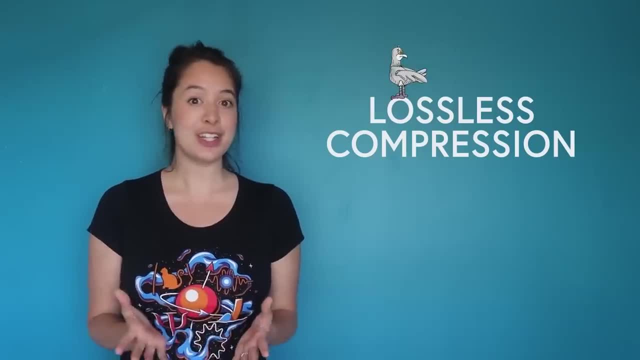 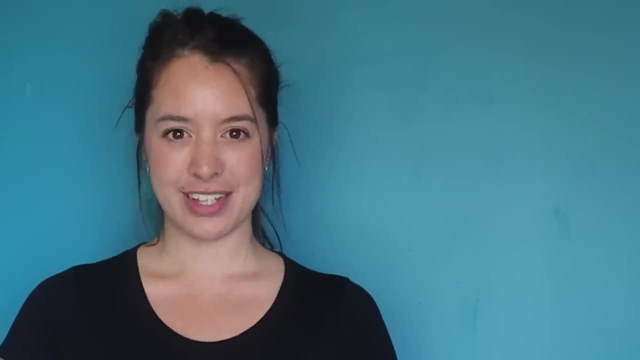 It's just transformed. Lossless compression is really useful for things like text files, where the original file needs to be replicated perfectly. So here's a question for you: Can you write a computer program that losslessly compresses any set of data? 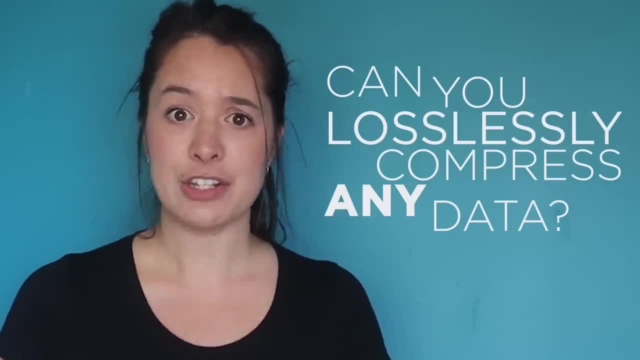 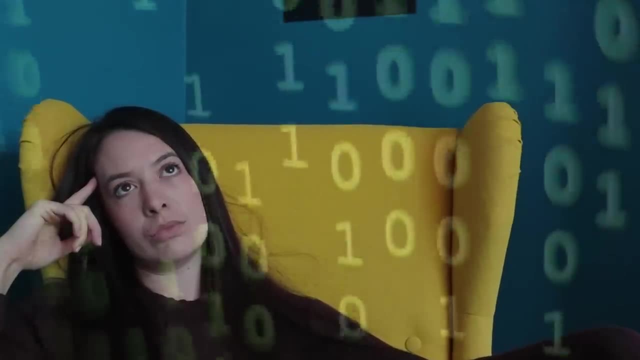 It sounds like a very big question. How would you go about answering it? Here's where my mind would go. Information compression is based on exploiting redundancies. Redundancies rely on there being some kind of pattern in the information. So as long as there's a pattern, 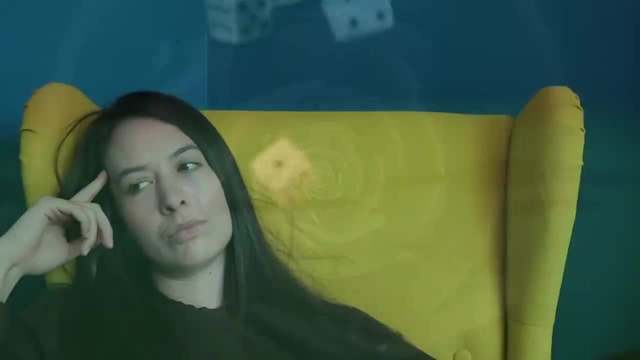 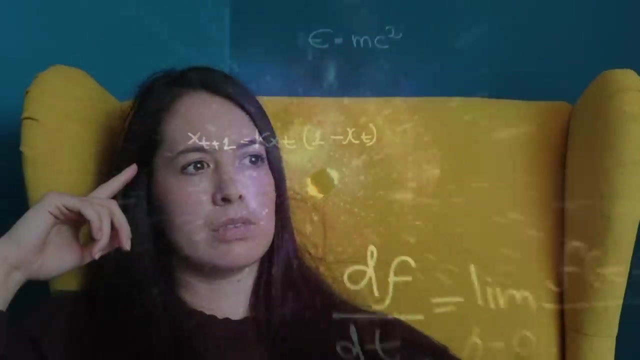 you should be able to compress the data. So then the question becomes: does true randomness exist? Maybe it's just that we're not clever enough to spot the pattern? A pattern's objectively real, or is everything merely information and our minds need to simplify? 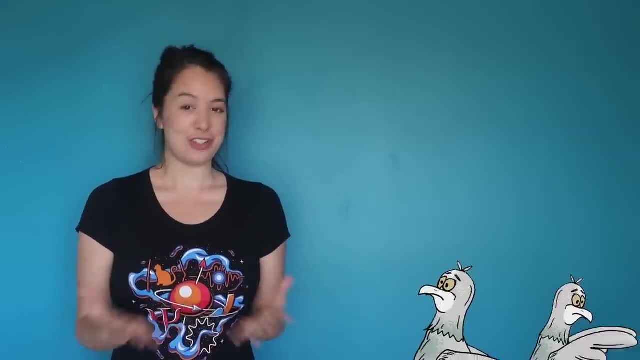 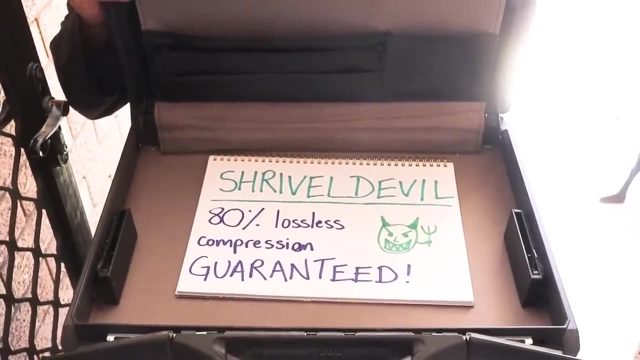 to make sense of the universe. But there's a much simpler way to answer this question, using the pigeonhole principle. Imagine a company claims that their new program, Shrivel Devil, can compress any file to 80% of its original size, then decompress it back to its original file. 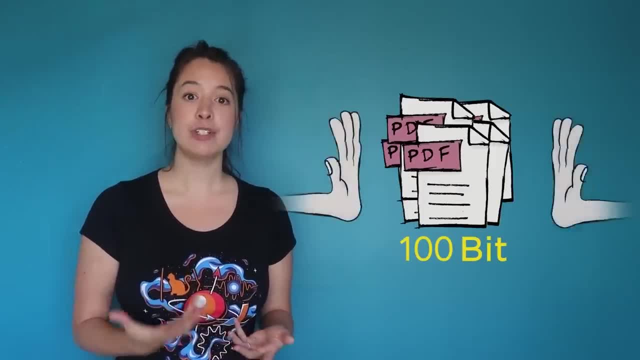 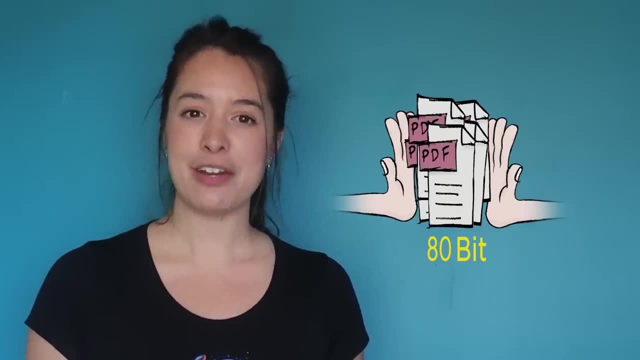 You've got a bunch of eBooks that are 100-bit files, so Shrivel Devil claims to be able to compress them all into 80-bit files. It doesn't sound so far-fetched, but here we invoke the pigeonhole principle. First, let's ask how many 100-bit files. 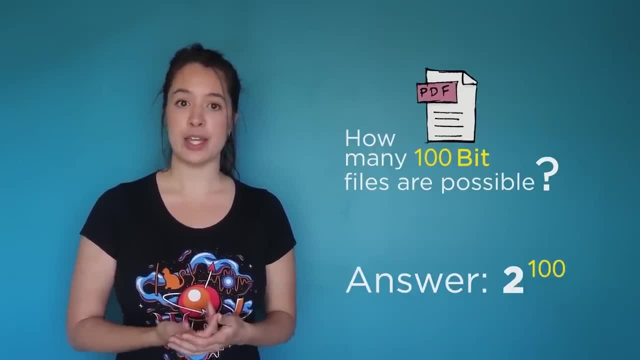 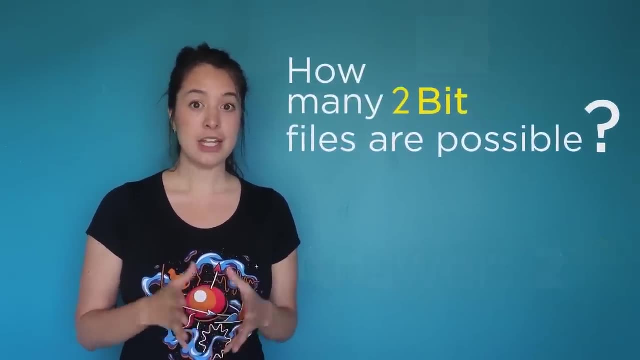 can we possibly have? A simple calculation shows that we can have two to the power of 100 of them. To see how I got this number, let's start smaller. How many two-bit files are possible? A bit can either be a one or a zero. 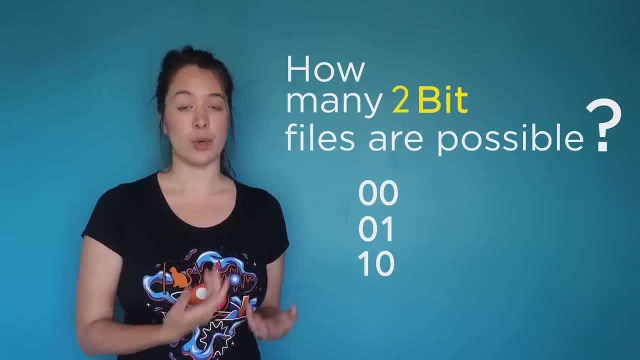 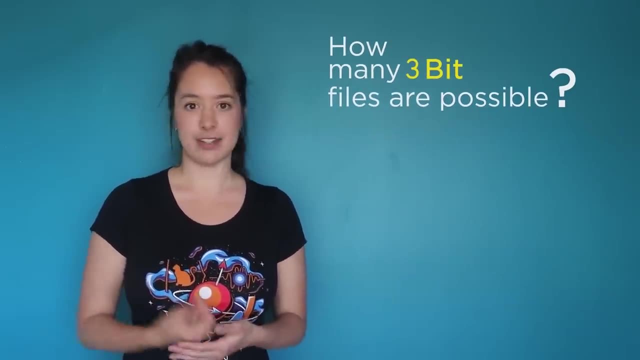 so we can have 00,, 01, 10, and 11.. Four possible files, which can also be expressed as two, to the power of two files. How many three-bit files can we possibly have? 000, 001, 010, 011, 100, 101, 110, and 111.. 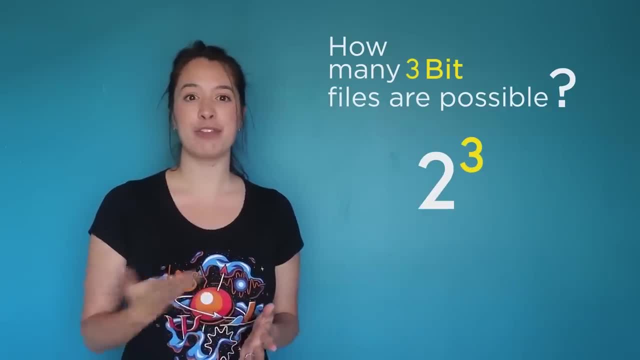 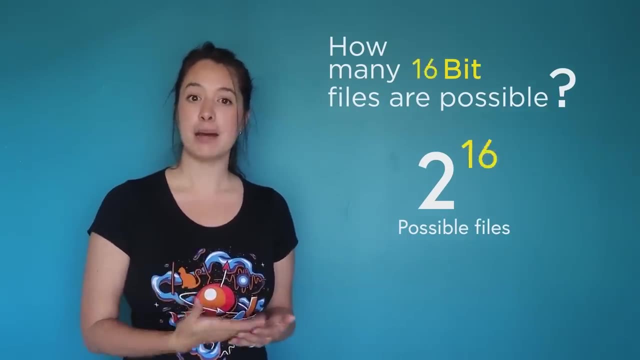 Eight different files, which is also expressed as two to the power of three. How many four-bit files? 16, or two to the power of four. The pattern is pretty obvious. For any number of n bits, there are two to the power. 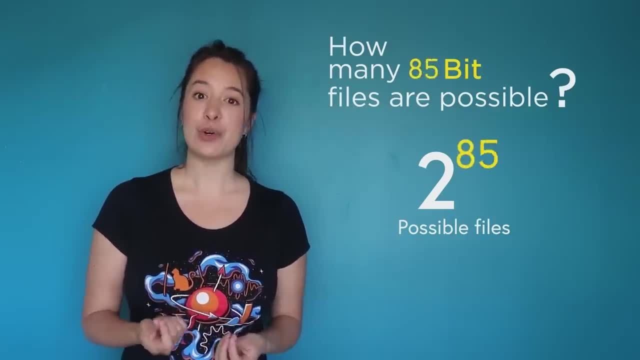 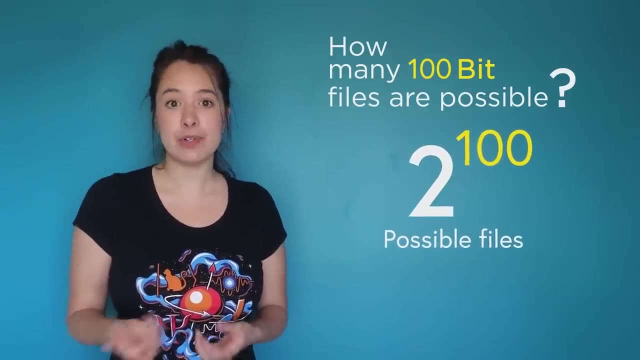 of n possible arrangements and therefore two to the power of n possible files. So the number of possible files we have with our 100-bit eBooks is two to the power of 100, and the number of possible compressed files of 80 bits is two to the power of 80.. 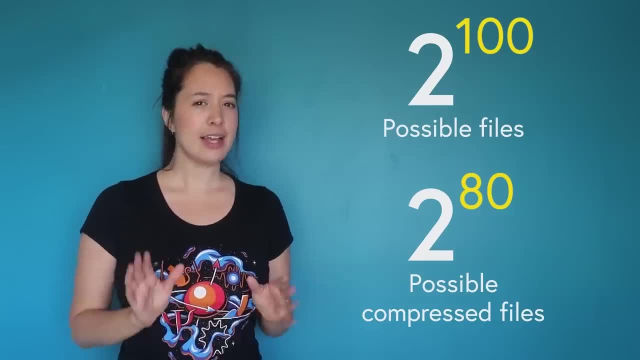 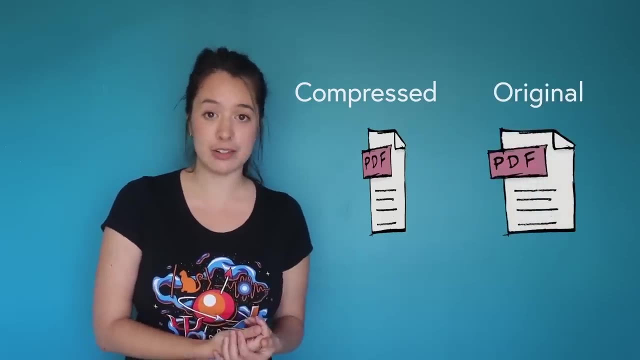 Now for lossless compression. to work, each compressed data file needs to decompress back to its original file. This means that each original file needs to map to exactly one compressed file and each compressed data file needs to be mapped to exactly one compressed file. and each compressed file needs to map back to exactly one original file. If two original data files are compressed into the same smaller file, how will that one smaller file expand into two different original data files? It won't. One will be lost. So how are we going to compress two to the power of 100 original data files? 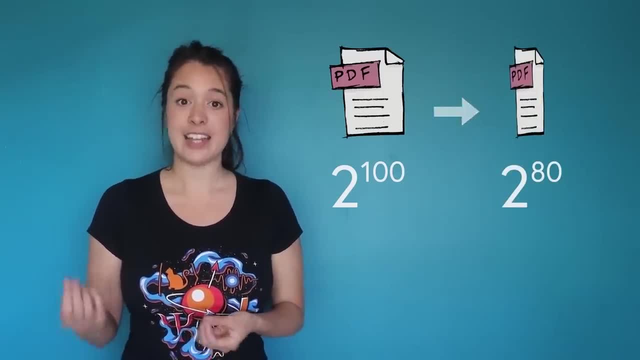 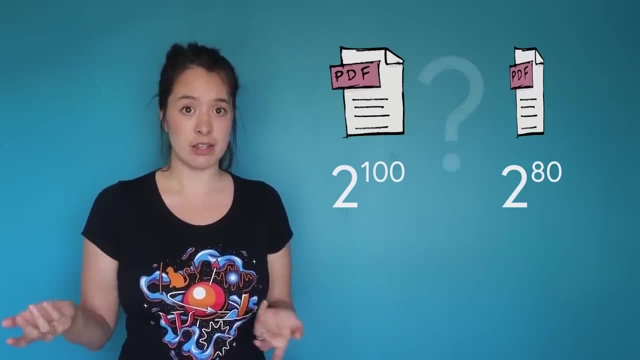 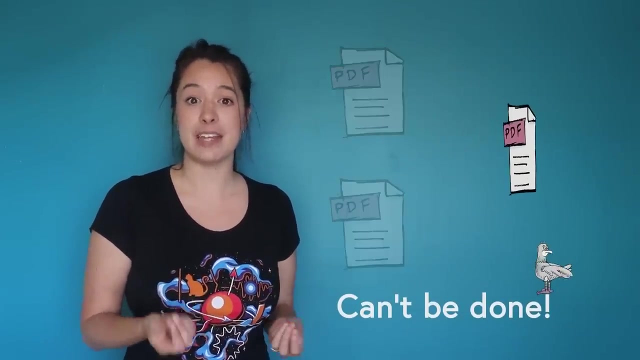 into two to the power of 80 compressed data files And then decompress two to the power of 80 files, back into two to the power of 100 files, without losing any files. The answer: We can't More than one 100-bit file is going to be compressed into the same 80-bit file. 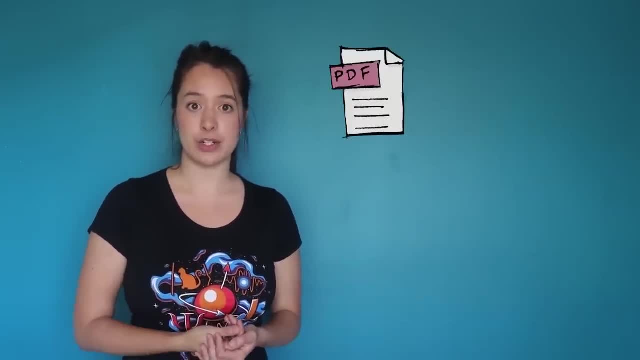 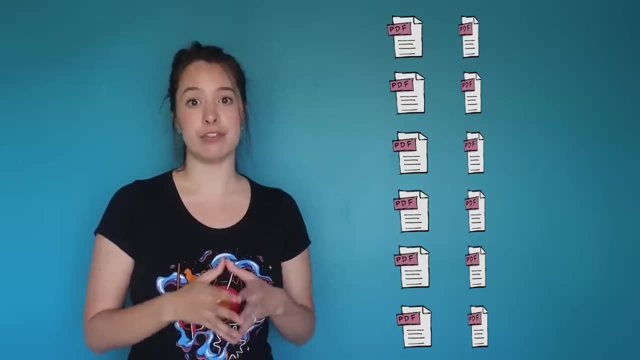 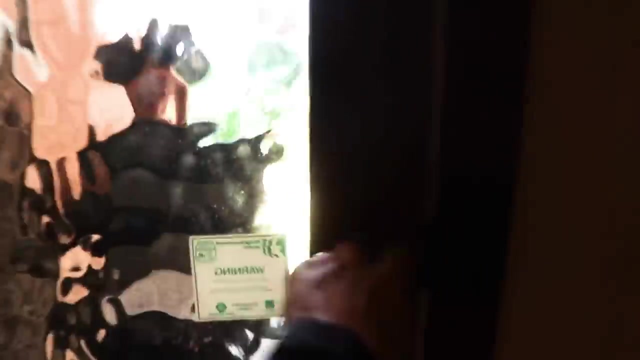 and therefore one of the files will be lost during decompression. For this compression program to work, each 100-bit file would need to be compressed into an individual 80-bit file, which the pigeonhole principle tells us is impossible. As tempting as it sounds, you'll have to pass on Shrivel Devil. 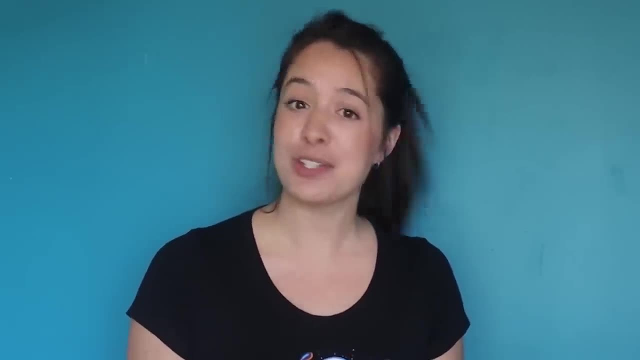 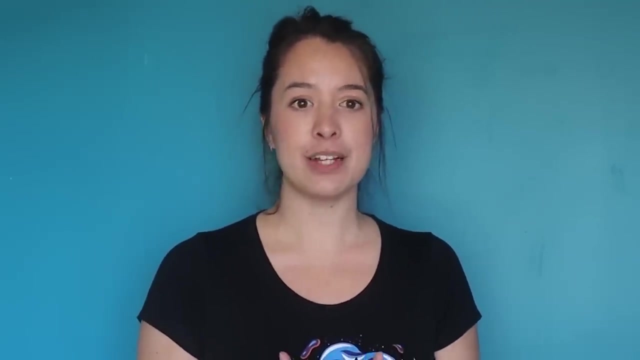 A program that losslessly compresses any file is impossible. It violates the fundamental rules of mathematics. I just think this proof is really clever because it's so simple and just not where my mind would have gone. You might be starting to see the unexpected power of the pigeonhole principle. 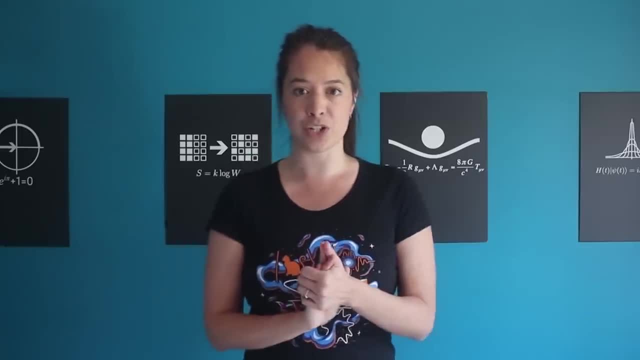 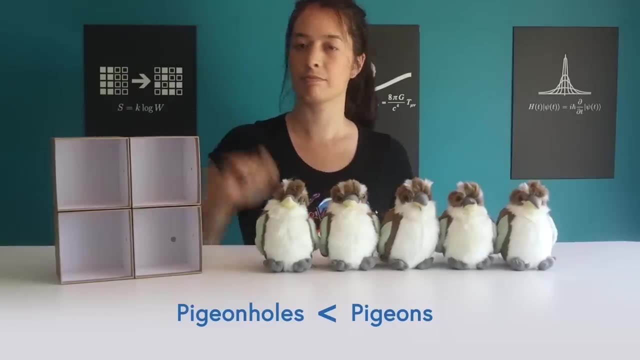 But what would happen if we extended it from a finite number of objects to an infinite number of objects? So far we've used it like this: If the number of pigeons is larger than the number of pigeonholes, we can't have a one-to-one. 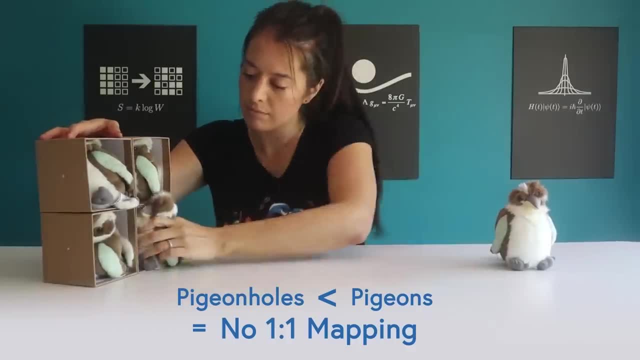 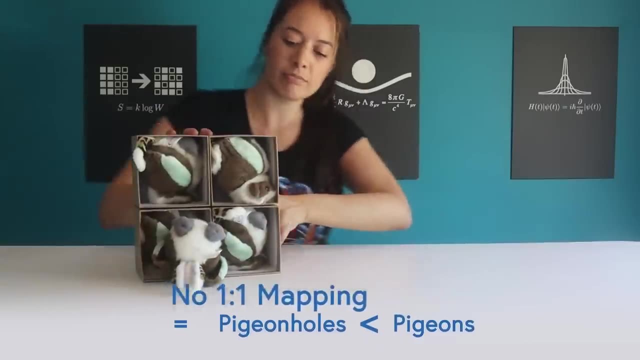 We can't have a one-to-one mapping between pigeons and holes. Therefore, we will always end up with at least one pigeonhole with two pigeons in it. But what if we flip this on its head? What if we use the fact that, if we can't have a one-to-one mapping between pigeons and pigeonholes, 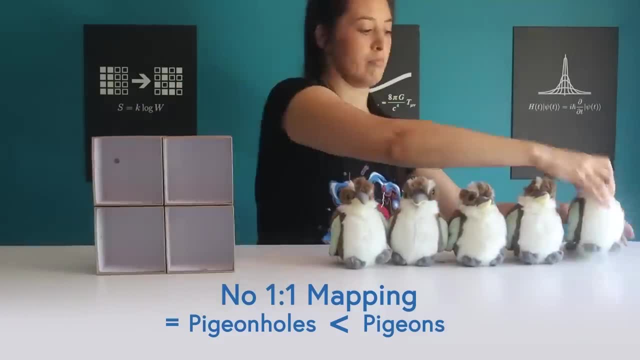 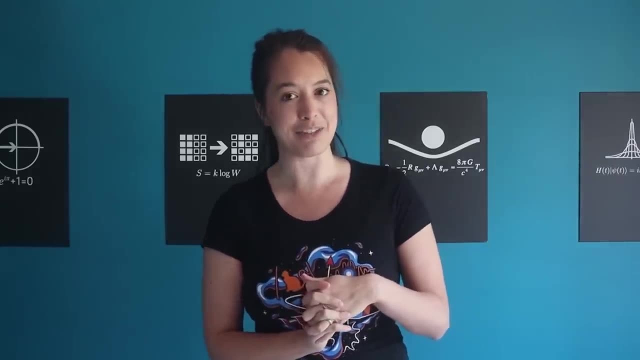 it means that the number of pigeons can't be equal to the number of pigeonholes. It doesn't sound like much of a difference, but by flipping the argument we can prove some pretty crazy things about infinity. Let's say that two sets of objects are the same size. 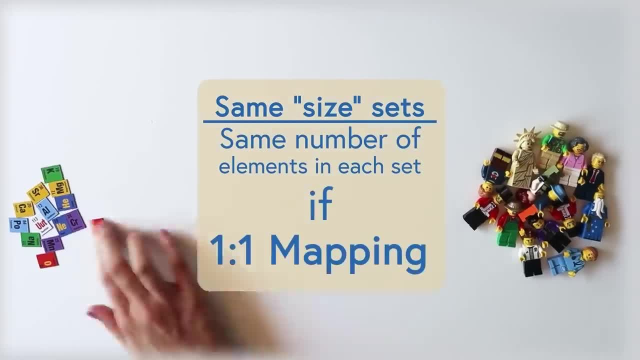 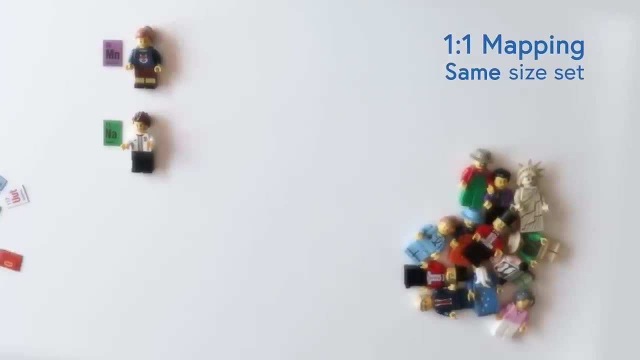 that is, they have the same number of objects or elements in them. if you can create a one-to-one mapping between every element in each set with no elements left over. But if we make a one-to-one pairing and some LEGO people are left over. 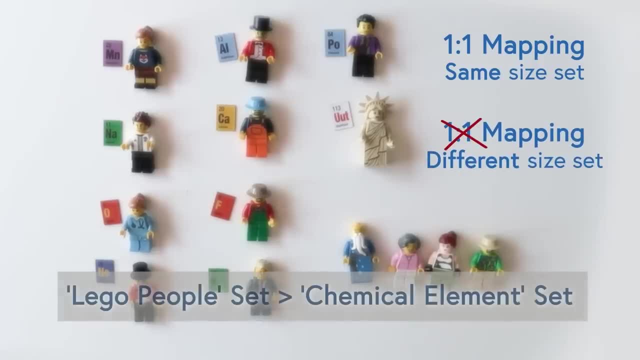 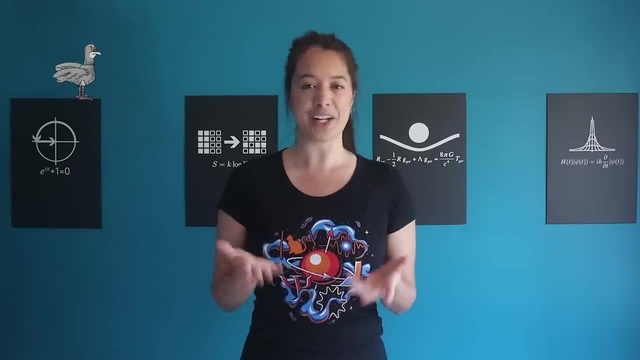 we know that we have more LEGO people than chemical elements. In math talk, we say that the set of LEGO people is larger than the set of chemical elements. This is pretty simple when it comes to finite sets, but things start to get weird when we extend this simple reasoning to infinite sets. 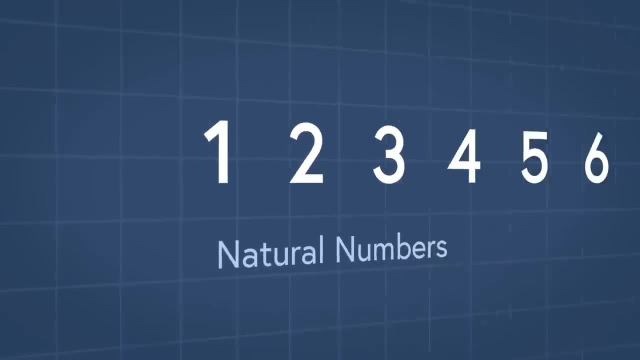 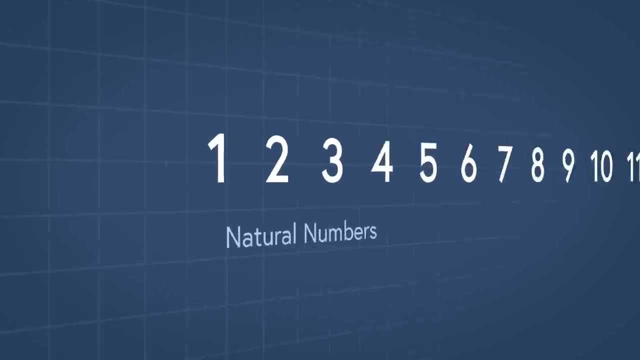 Take the set of natural numbers. These are the positive integers from one to infinity. There are infinitely many natural numbers, as we can count them forever and never stop. Now take all of the negative whole numbers, which are also infinite as they extend to negative infinity. 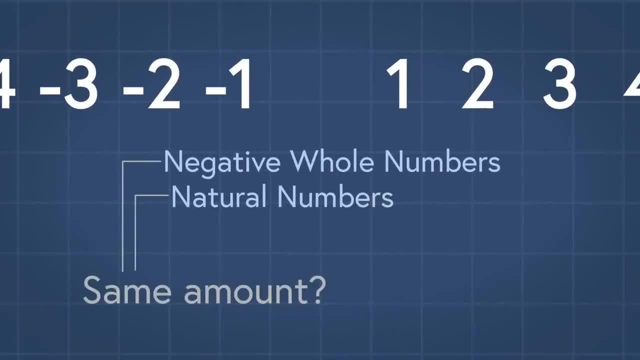 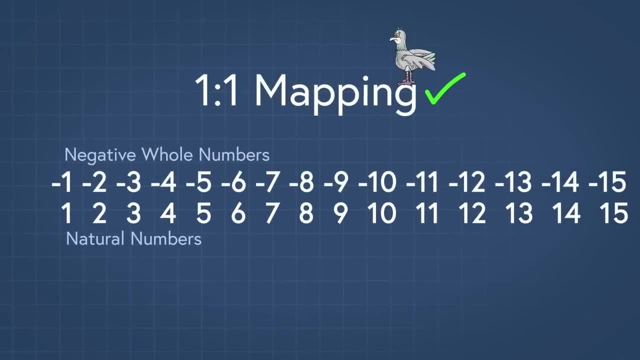 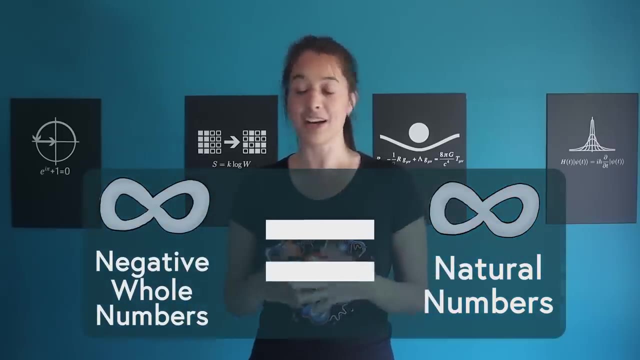 Are there the same number of natural numbers as negative whole numbers? Unsurprisingly, yes, We can map every natural number to a corresponding negative whole number. According to our one-to-one mapping argument, the infinity of the natural numbers and the infinity of the negative whole numbers are the same size. 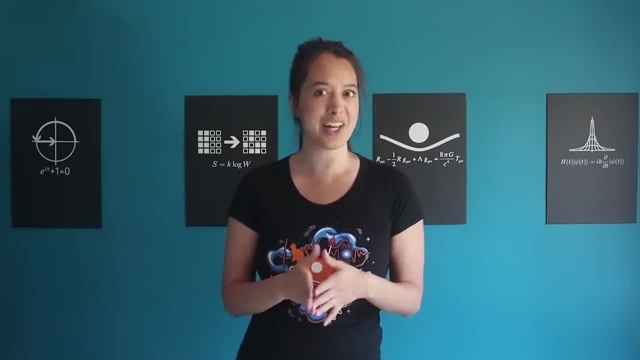 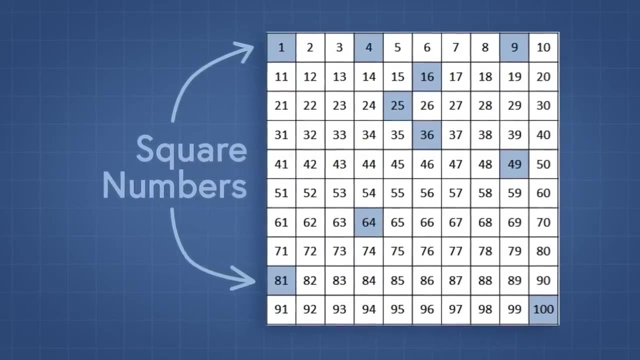 What about the infinity of the natural numbers compared with that of the square numbers? Square numbers make up only a small part of all of the natural numbers, so you might think that the infinity of the natural numbers is larger than the infinity of the square numbers. 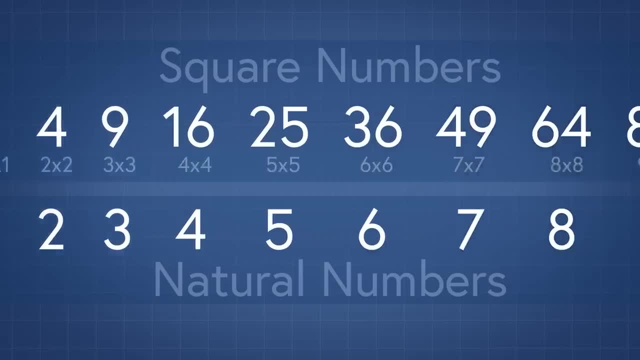 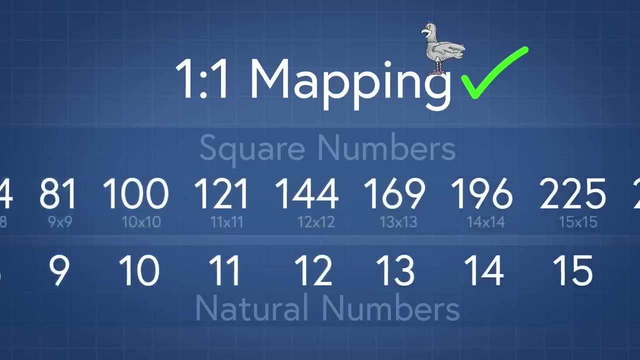 But let's try a one-to-one mapping idea. We can see that for every natural number there's a corresponding square number. This is more surprising. The infinity of the natural numbers and the infinity of the square numbers are actually the same size. 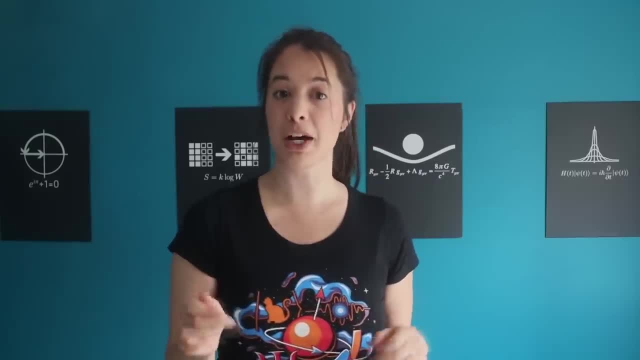 This is a pretty weird property of infinite sets: A smaller part of a set, a subset, can be the same size as the set itself. In math talk, when two sets have the same size, we say that they have the same cardinality. 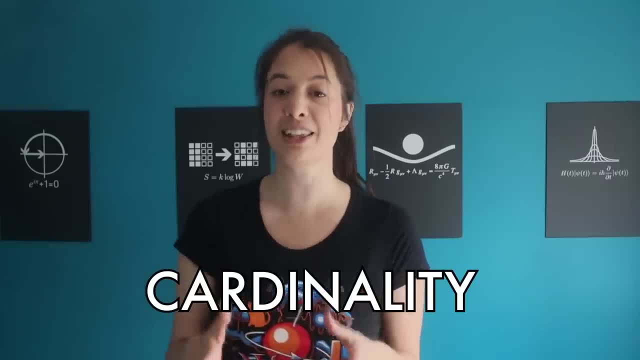 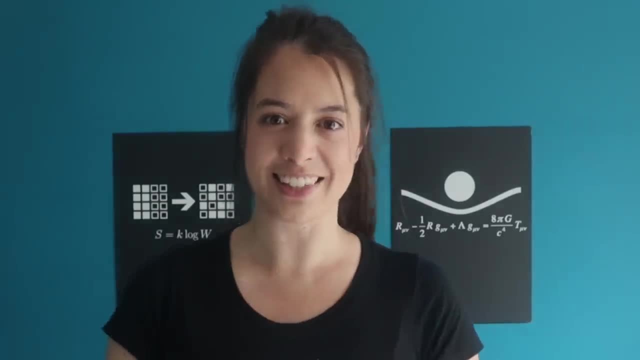 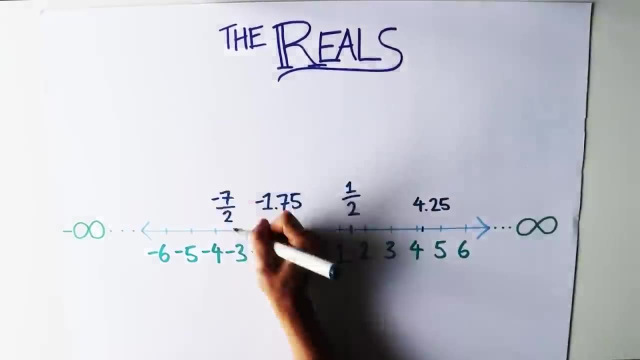 The cardinality of the natural numbers, the infinity of the negative whole numbers and the square numbers is represented by this symbol and called aleph null. So are there infinities bigger than aleph null? Take the set of real numbers. These include all the whole numbers, rational numbers and irrational numbers. 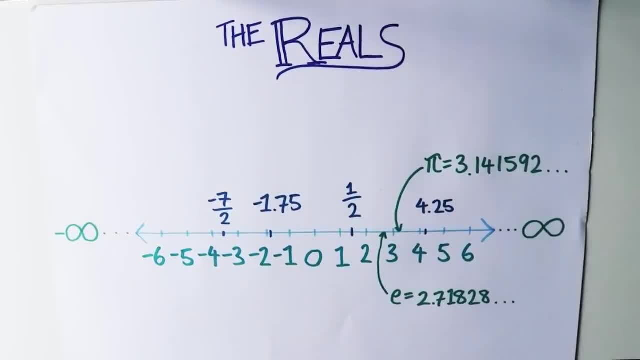 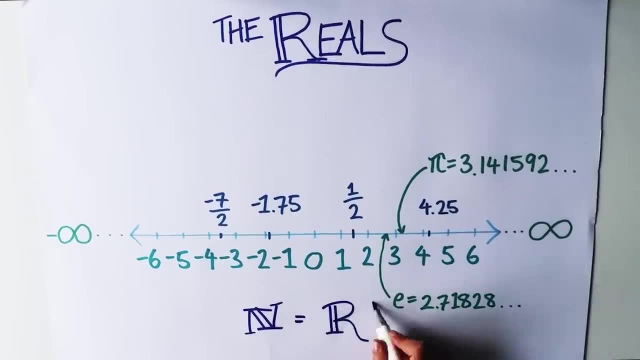 numbers that cannot be expressed as a ratio. They make up all of the numbers on the continuous number line. Are the infinity of the natural numbers and the infinity of the real numbers the same size? We can answer this question by saying that the infinity of the natural numbers and the infinity of the real numbers are the same size. We can answer this the same way we answered for the other sets of numbers, by seeing if we can create a one-to-one mapping. To keep things simple, we're going to limit the reals to just those between 0 and 1, for now. 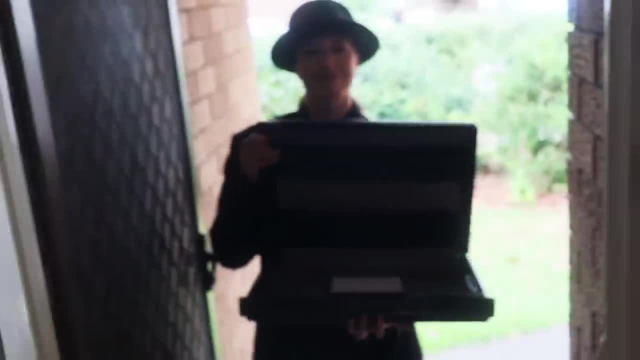 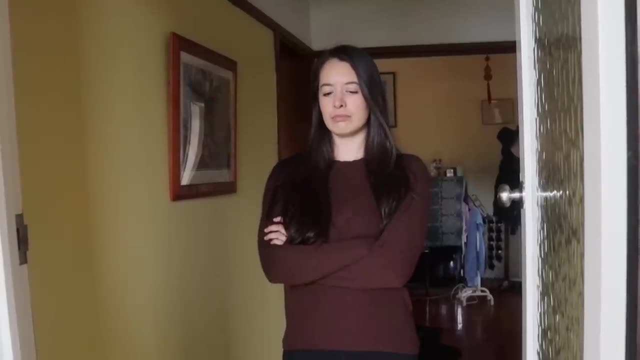 So where do we start? But wait, someone knocks on your door claiming that they have already made a one-to-one mapping. This person looks shifty and you don't know if you can trust them. But can you prove them wrong? They claim that they have mapped every real number to a natural number. So to prove them wrong, you need to come up with a new real number that definitely isn't on their list. Can you do it? You take the first decimal of the first number and add one. Now you take the second decimal of the second number and add one. 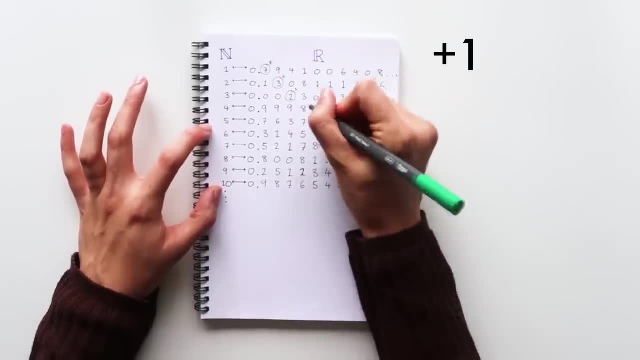 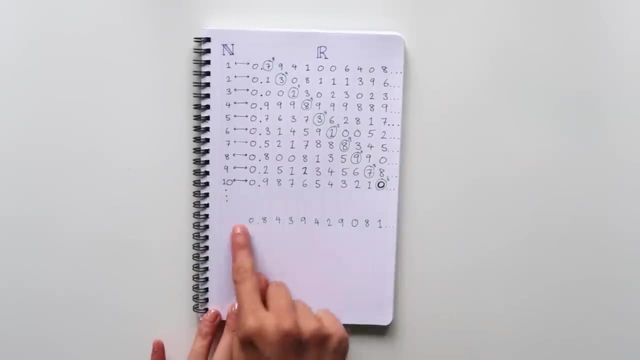 Now you take the third decimal of the third number and add one. You keep doing this for every single number on their list and you make a new number out of it. Was this number on their original list? Well, it's definitely not the first number. 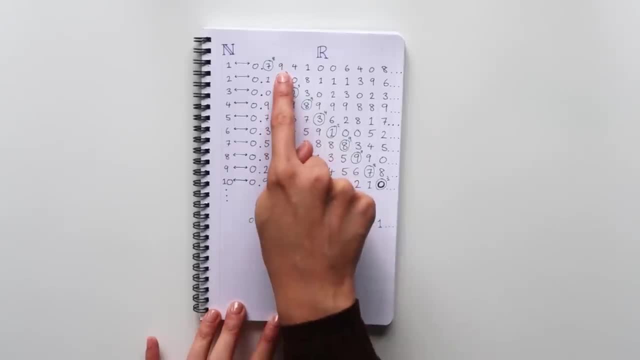 because the number in the first decimal place is different, And it's definitely not the second number, as the number in the second decimal place is different. You can make this argument for every number. It's definitely not the one millionth number, because the one millionth decimal place will be different. 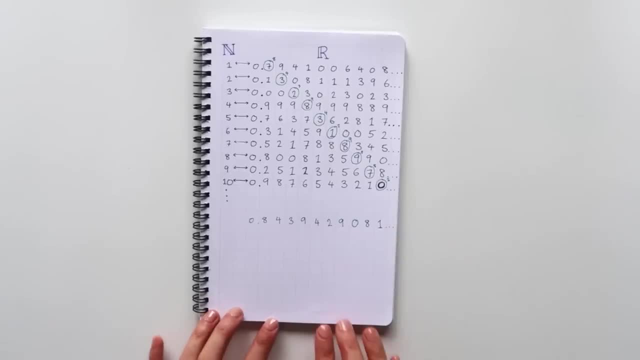 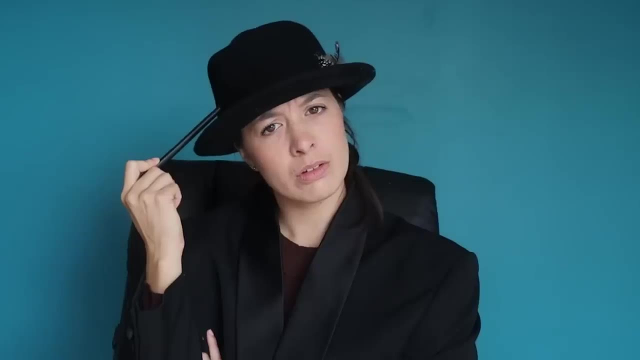 Even though there were an infinite amount of real numbers on this list, you've managed to come up with a number that wasn't on the list. Therefore, the claim that there was a one-to-one mapping between every natural number and every real number. 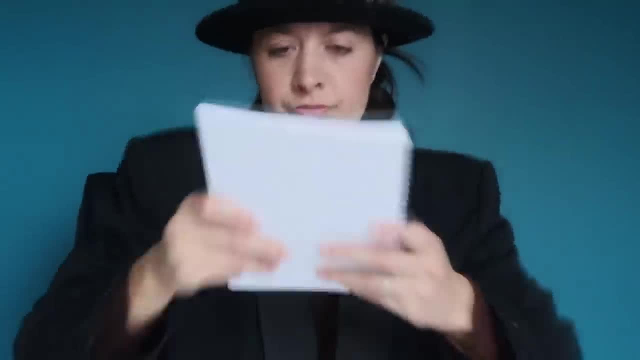 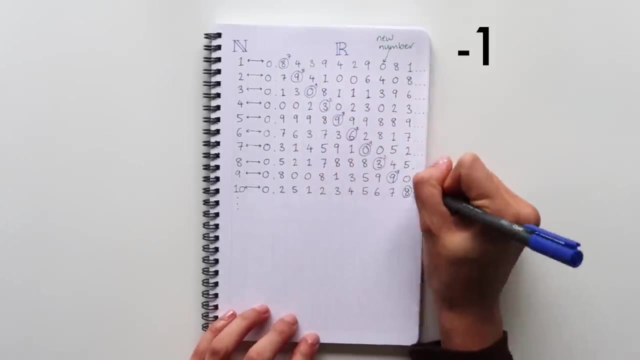 must have been false, But our person's not giving up. They just add the new number to the list. Problem solved, right? No, you're onto them This time. you subtract one from every subsequent decimal place. This number also wasn't on the list.